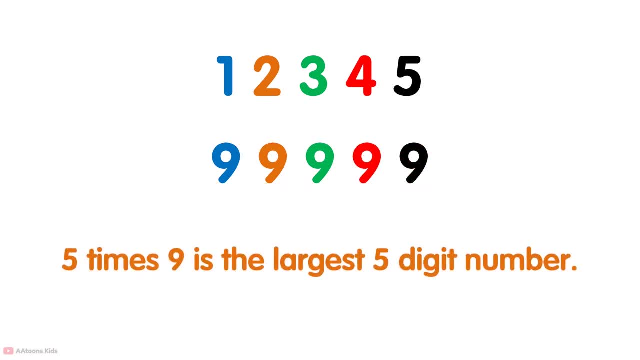 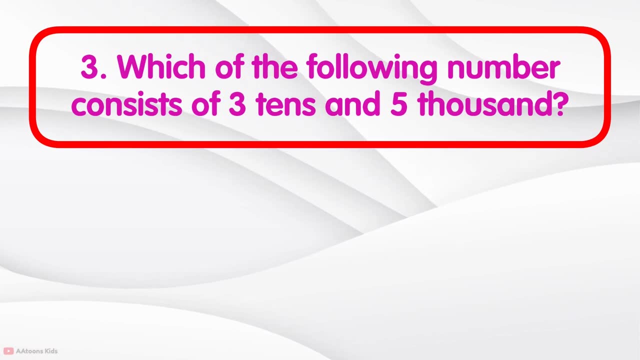 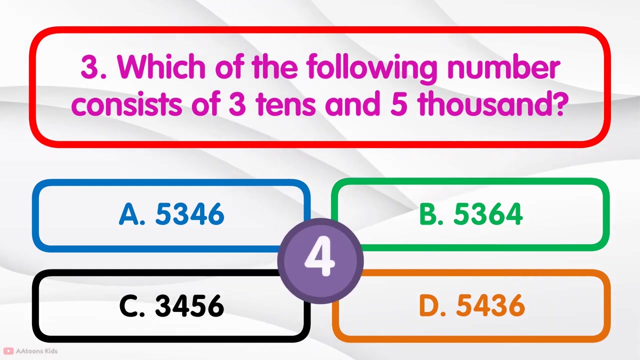 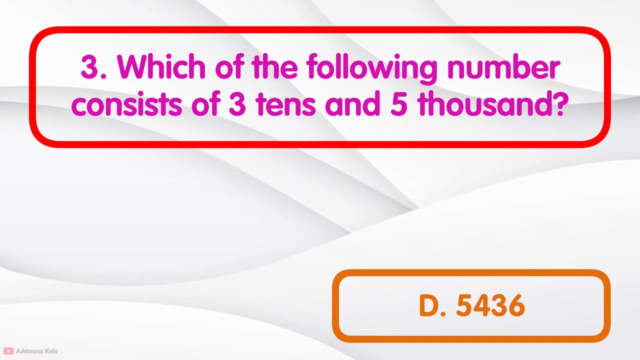 5 times 9 is the biggest 5 digit number. Which of the following number consists of 3 tens and 5,000?? 5,436 contains 3 tens and 5,000.. 3 in the tens place and 5 in the thousands place. 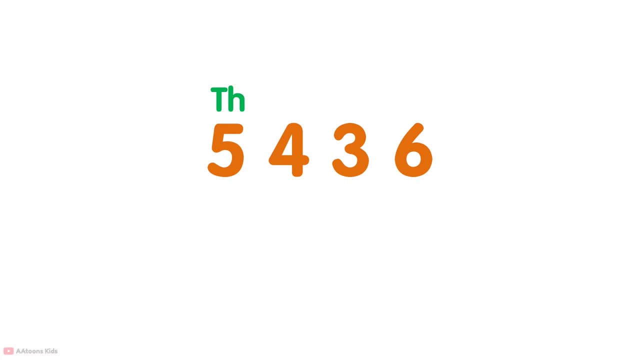 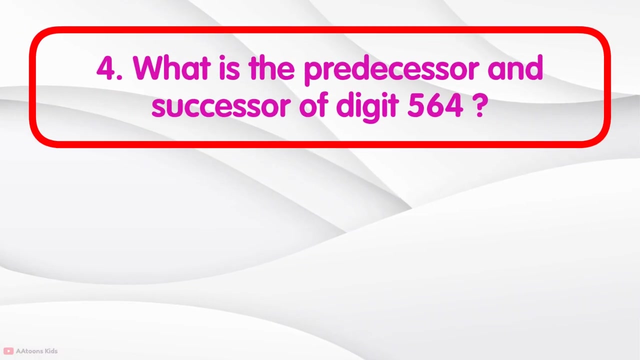 5 is in the thousands, place 4 is in the hundreds, place 3 is in the tens place And 6 is in the units. place 5 is in the thousands place and 3 is in the tens place. What is the preceder and successor of digit 564?? 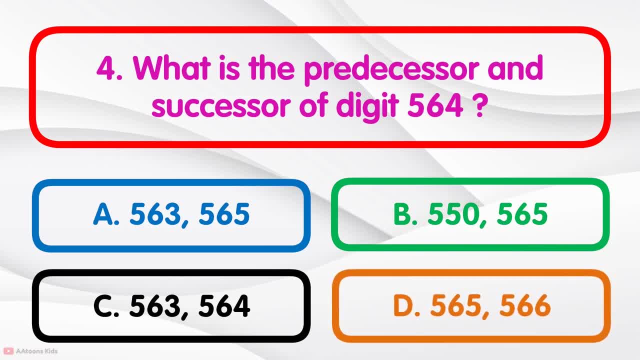 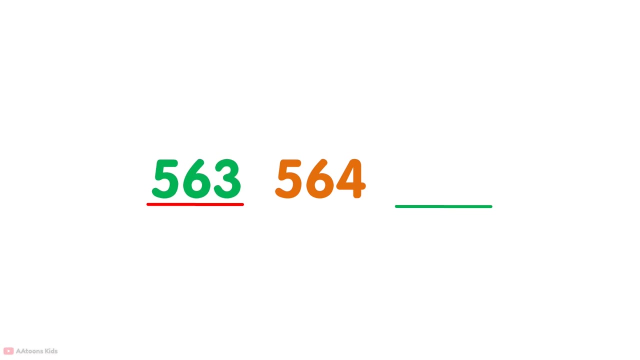 5 is in the tens place. What is the preceder? Option A, No preceder and 565.. 5 is in the tens place. Option C is 87.. Option D is null. Option A is 82.. Option D, C and A are the most frequent. 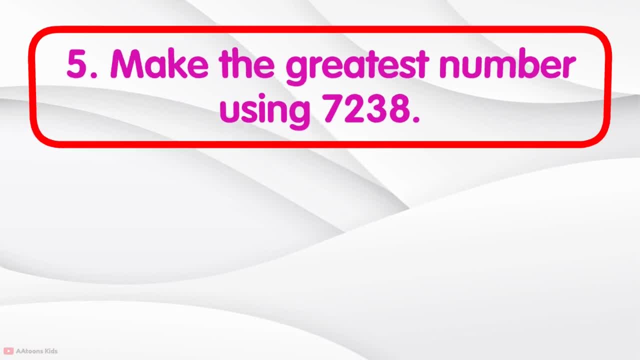 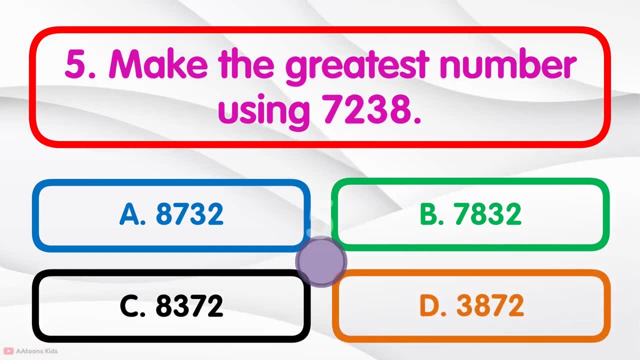 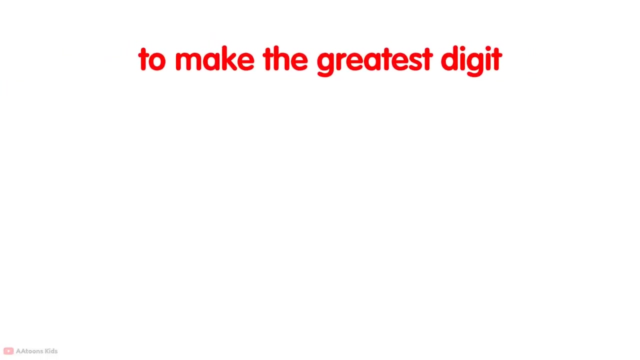 Successor means after the number. Make the greatest number using 7238.. 8 7 3 2. 8 7 3, 2 is the greatest number. To make the greatest digit number, simply arrange these numbers in descending order. 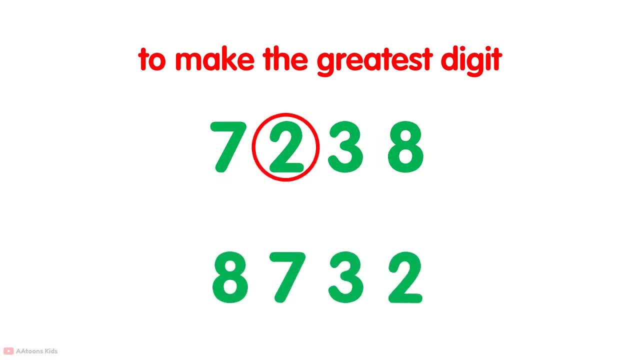 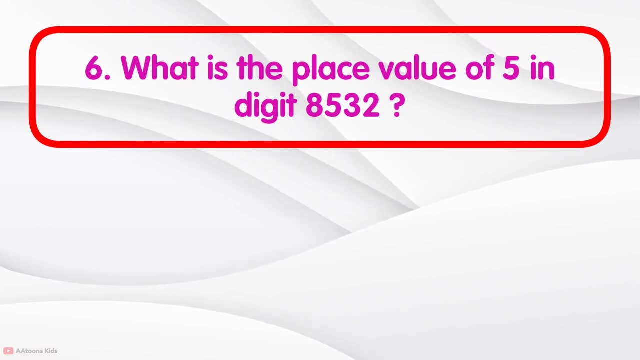 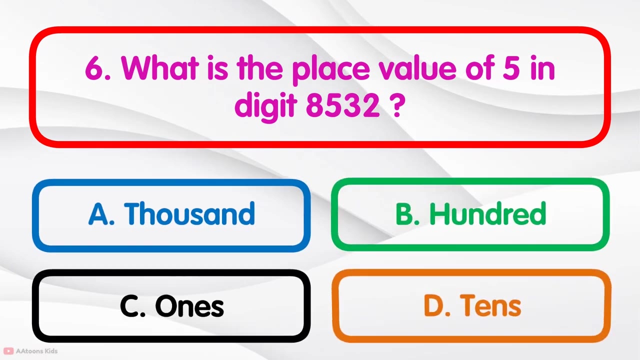 8, 7, 3, 2, 8732. What is the place value of 5 in digit 8532?? 8, 7, 3, 2. 8, 7, 3, 2, 8732. What is the place value of 5 in digit 8532?? 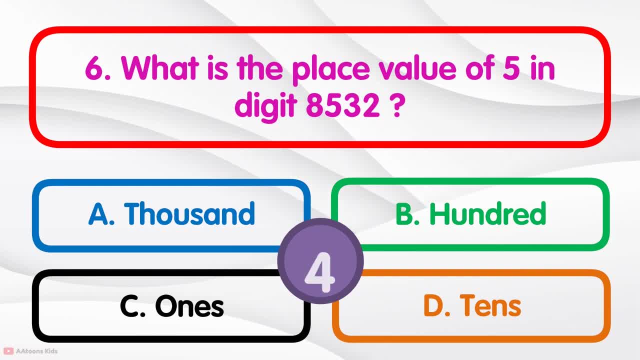 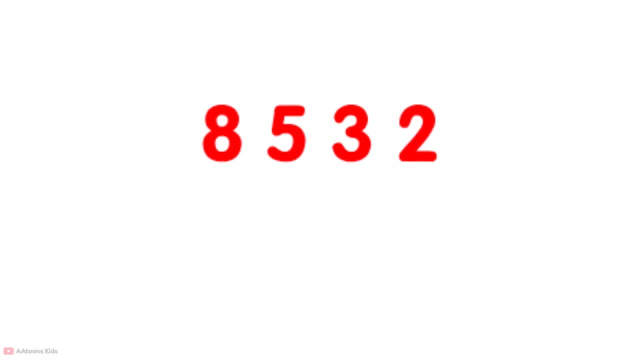 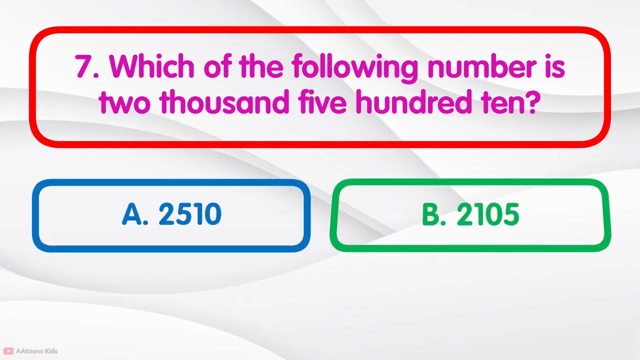 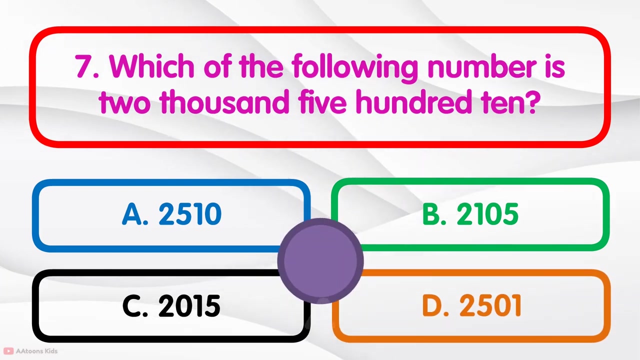 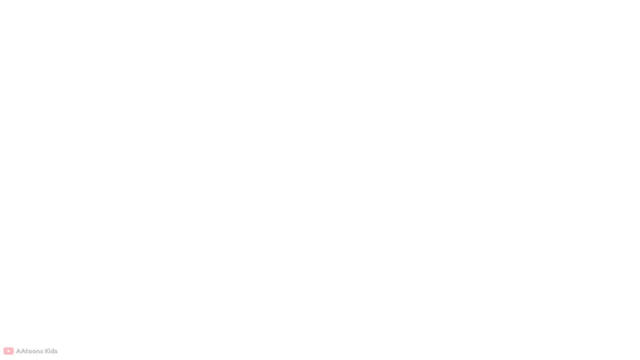 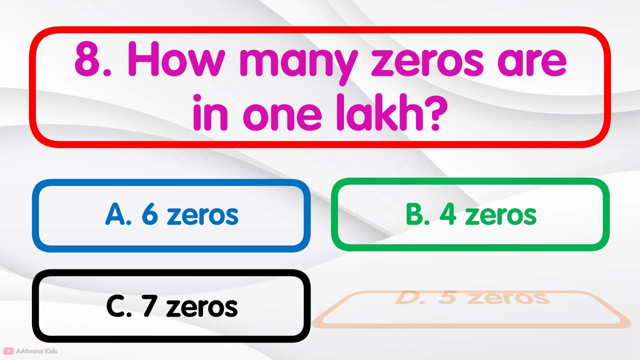 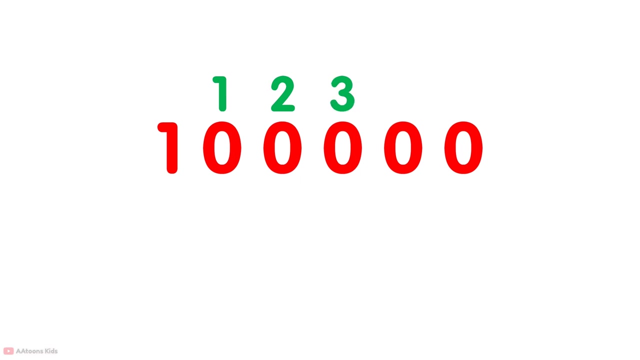 Number CB: Hundredth place. Ones, tens, hundreds, thousands. 5 is in hundredth place. Which of the following number is 2510?? Option A is 2510. How many zeros are in 1 lakh? 5 zeros 1, 2, 3,, 4, 5. 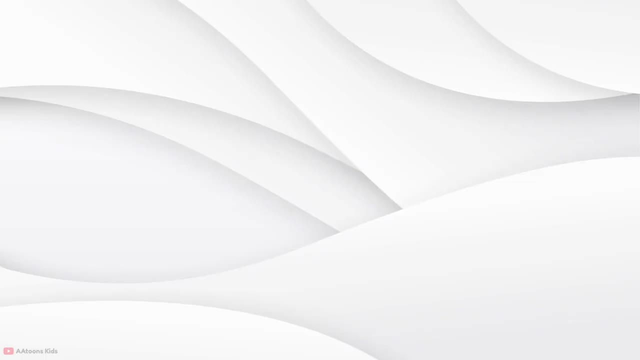 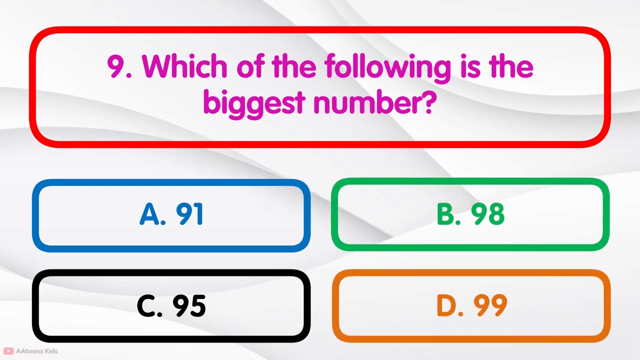 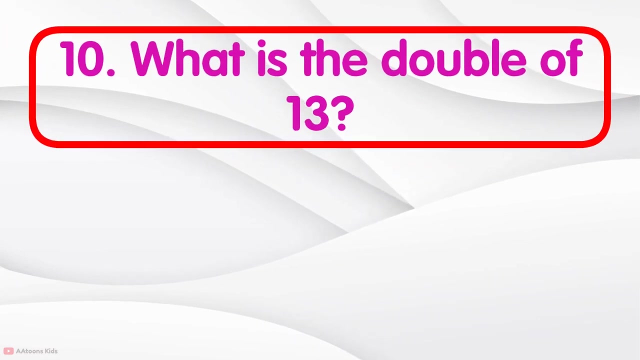 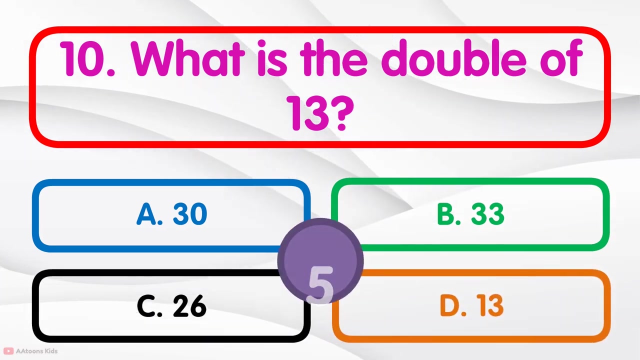 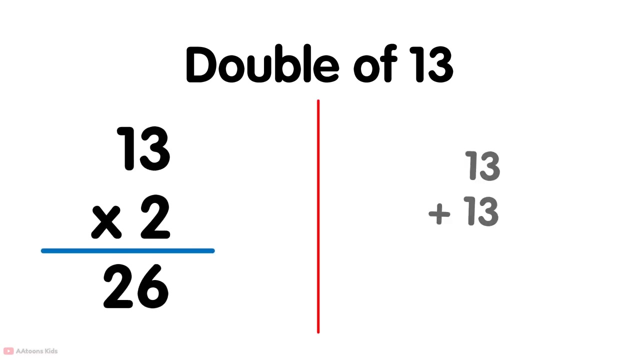 1 lakh has 5 zeros. Which of the following is the biggest number? Option D: 99th is the biggest number. What is the double of 30?? 26th is the double of 13. to double any number, simply multiply the number by 2 or add the number to.